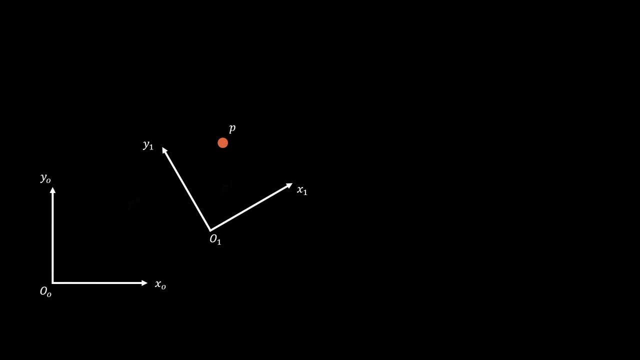 and we want to find this point's coordinates relative to frame 0. This operation combines a translation of distance and a frame rotation, So we have a representation for the rigid motion. but we want to turn this summation operation into a singular linear matrix operation because it'll 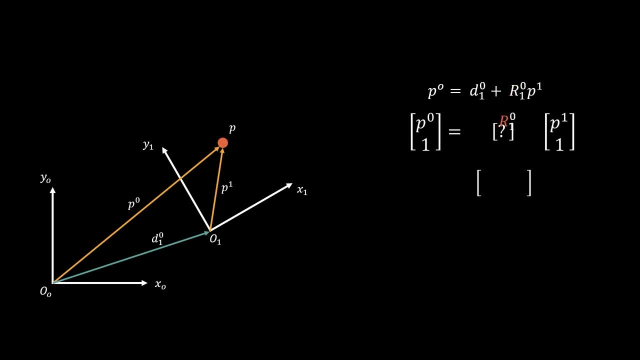 help a lot with frame transformation transformations later. So with some rearranging and padding we can rewrite this transformation as a singular matrix to represent the translation and rotation of the point. And this 3x3 matrix is known as the homogeneous transformation matrix and is a linear representation. 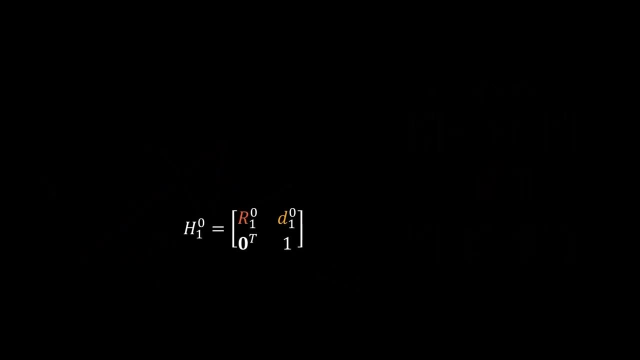 of rigid bodies. So let's break down what the homogeneous transform matrix represents. We expand it out For the 2D homogeneous matrix. the first two rows and columns represent the rotation component and the third column represents the displacement. The homogeneous matrix can 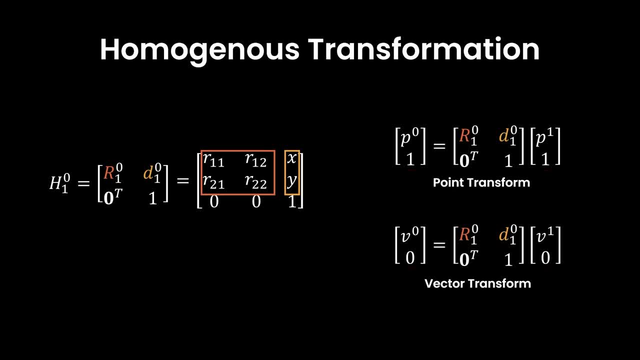 be used to transform points and vectors. Notice the difference in the last columns of the points and vectors. Vectors, which represents the difference between points and do not depend on frame location, have a zero as the last value in the column, and points have a one. 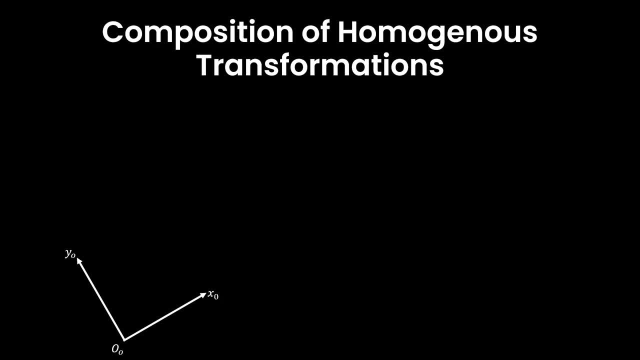 to represent the translation component, So we can build out multiple compositions. We can use the compositions of homogeneous transforms to represent multiple transformations. First we start with the rotations from frame 0 to 1, then the translations from frame 1 to 2.. To get the transforms of frame 0 to 2, we can multiply the two homogeneous transforms. 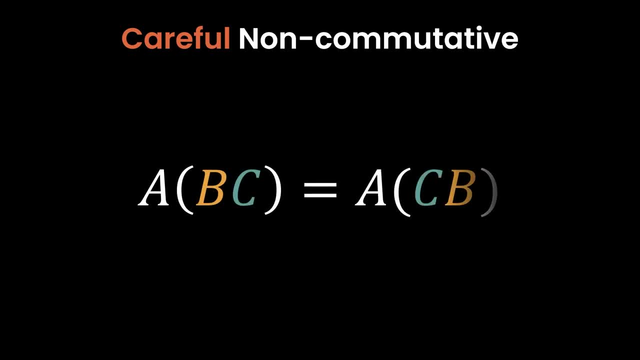 together. One thing to be wary of is that the compositions of homogeneous transforms are not commutative. That means that changing the order of multiplication doesn't give the same solution. So an example of this is shown with these frame transformations. Translations and then rotations doesn't allow us to think about. 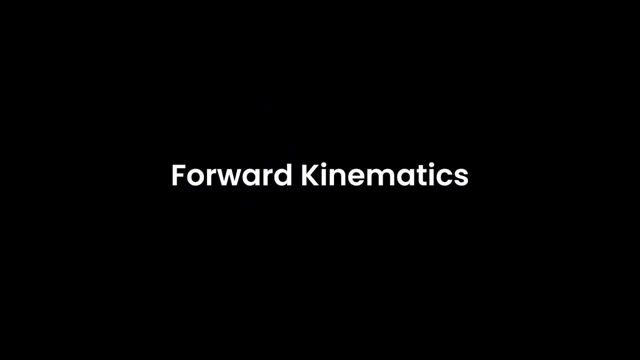 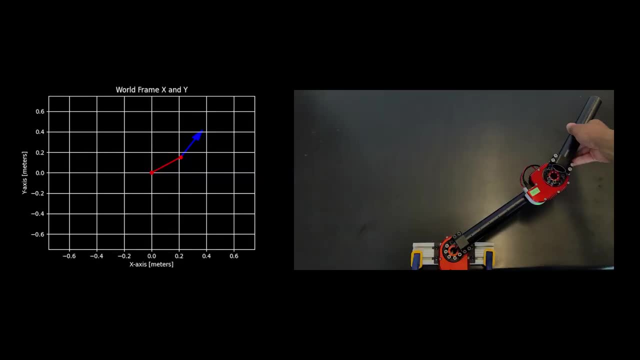 each product from its outstanding originality. The main reason for learning of this rigid body motion transform was for easier representation for forward kinematics. Forward kinematics is the process of going from the robot joints spaceneto last a task base or where the end effector would be in the world. 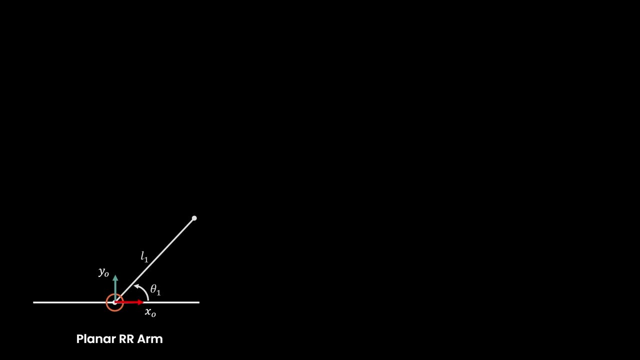 Prof空born Reposterk Haynes was the director of Midas for the introduction to the attacking. The simplest case is the planar 2-degree-of-freedom open-chain arm with known link lengths. The number of joints of the manipulator determines the degree of freedom of an open-chain manipulator. 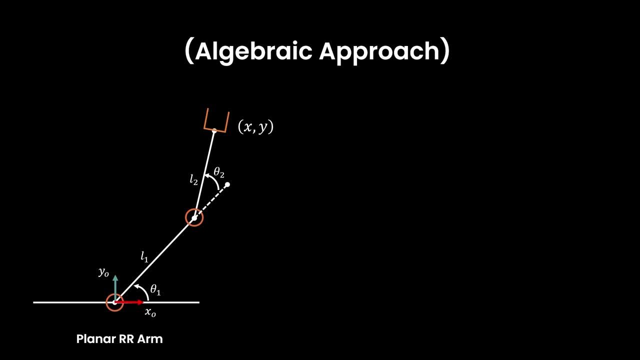 First we're going to analyze this from a complete algebraic perspective To get a formula for the robot: joint angles to the robot task space. we can build out the robot as simple triangles. This visual makes it simple enough to compute the task space and effective position from. 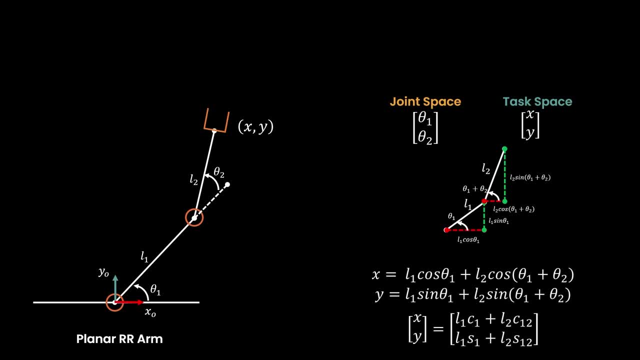 the triangles to get the x and y position relative to the robot joints, And then we can rewrite this position as a matrix with simpler notation. Now let's find this end-effective position using the information we just learned. With the homogeneous transforms of frames, the forward kinematic can be constructed by: 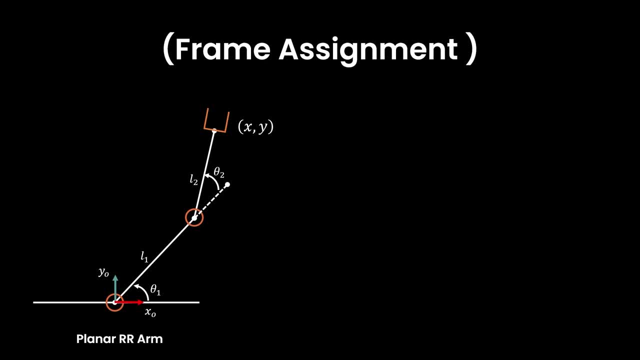 composing the rigid motion due to the individual joints. So we have four frames that represent the motion of the robot relative to the base. These four frames are the rotation due to joint 1.. The translation of rigid link 1,. the rotation of joint 2, and the translation of link 2.. 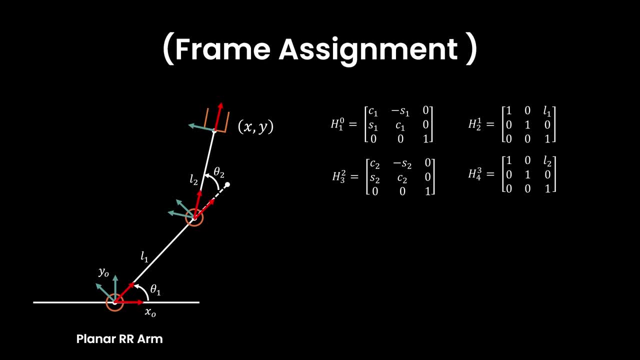 To compute the configuration of the end-effector relative to the base frame, we concatenate the rigid motions of the adjacent frames. Doing the matrix multiplication will yield a homogeneous transform that represents the final end-effector frame. The last column will yield the end-effector position. 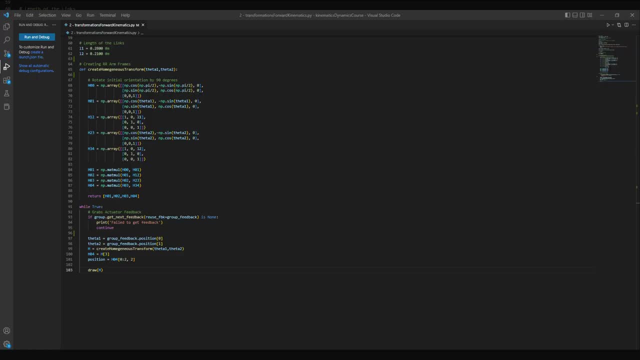 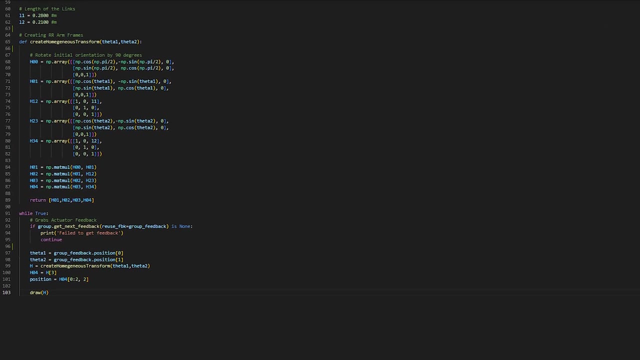 This is the same as we saw with the algebraic calculation. So look at an example of this. In Python, using Hebi hardware and API, we can calculate the end-effector position by initializing the link lengths, creating a function to calculate the homogeneous transform. 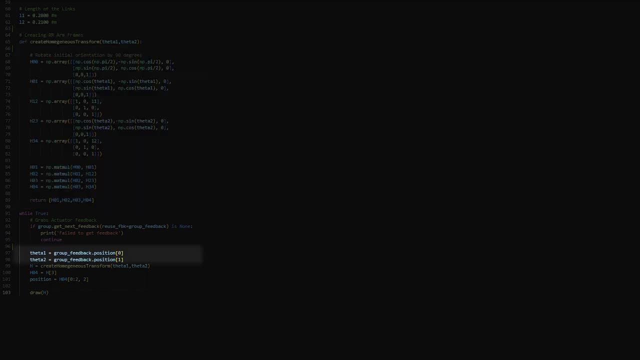 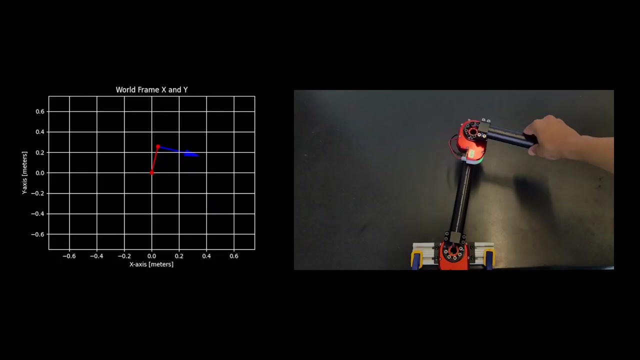 if we know the angles of the actuators constantly getting feedback from the robot position, and then final position can be pulled out with some matrix indexing. So this is me moving the 2 degree of film arm and output plot of the arm's updated position. 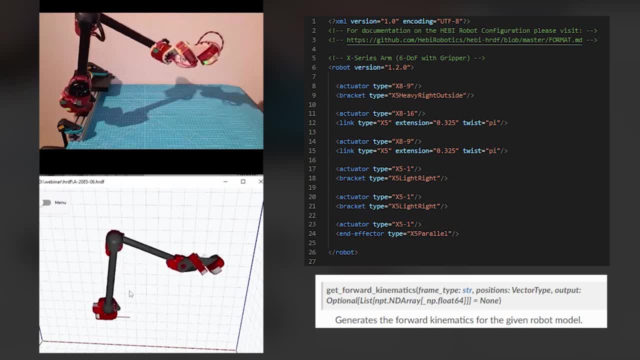 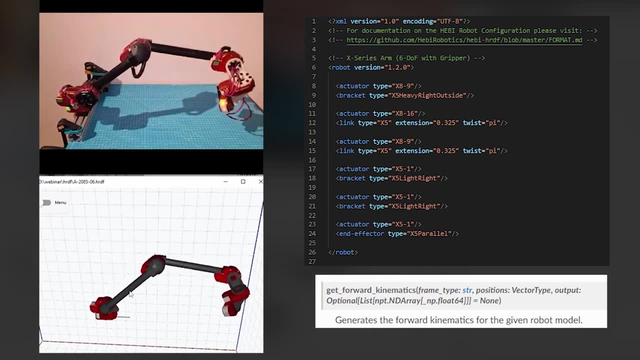 We have libraries that make it easy to build any open-chain robot. Here's the API calling the forward kinematic function with an arm built out in text formatting. So thanks for watching and visit Hebi Robotics to learn how our products can help with robotics. 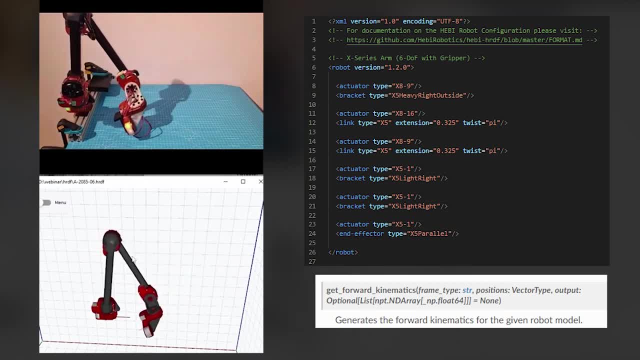 research and be using this tool for robotics development and education.